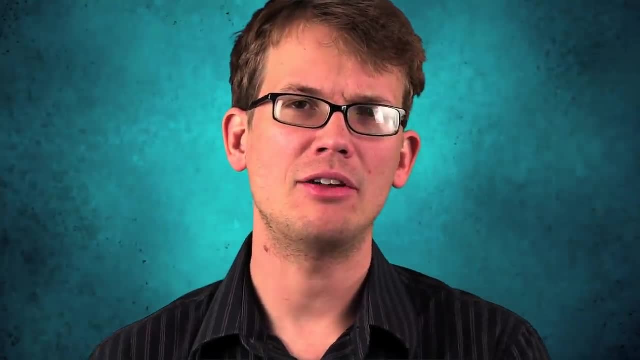 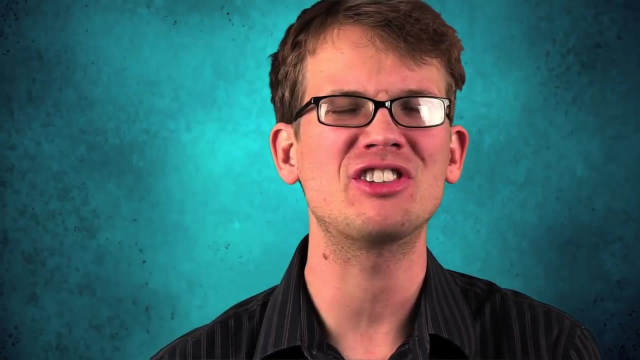 So I assume you know that there's a lot of people on this planet. As of last week- Wednesday I think- was when we turned over to seven, Nobody knows. but nobody knows exactly how many people there are. It's kind of hard to keep track. It's a big planet. 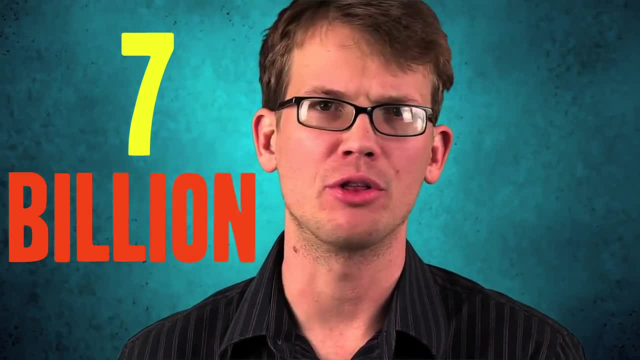 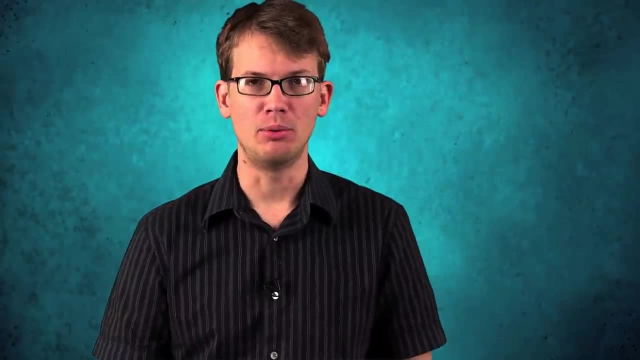 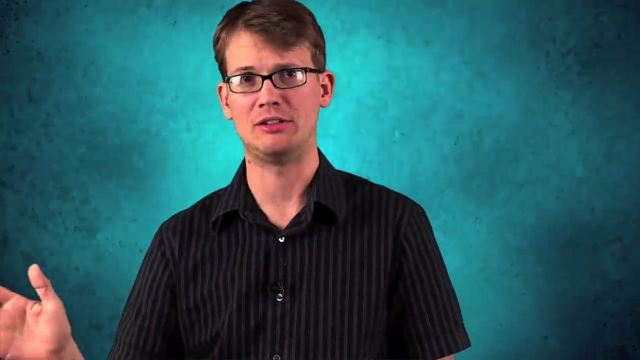 But there are about seven billion people on the Earth right now And they keep getting born all the time. In fact, for every two people who die, about four are born Every second. there are about four babies introducing themselves to this world and there are less than two people saying goodbye to it. 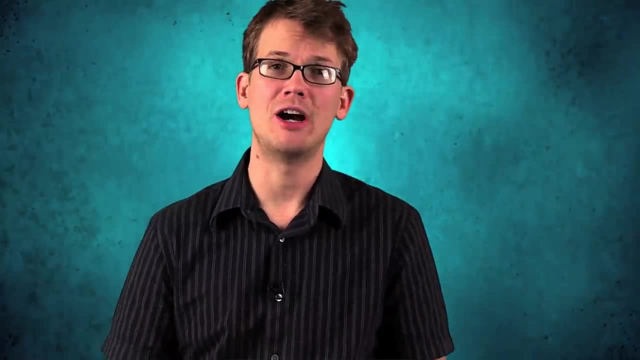 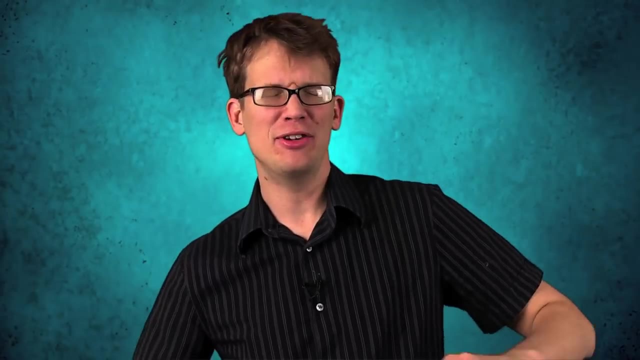 So easy math here. Our world's population is growing by about 2.5 people per second And as a reminder of this, during this video I'm going to have 2.5 ping pong balls being thrown at me every single second throughout the entire rest of the video. 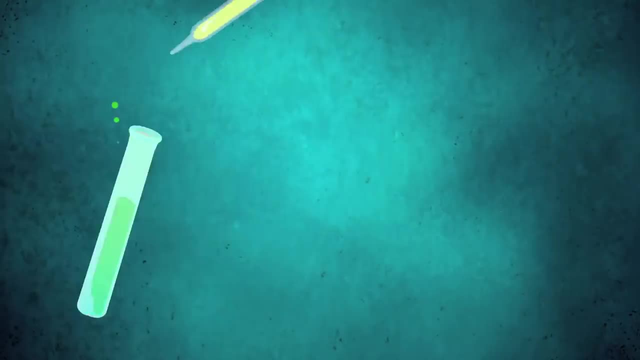 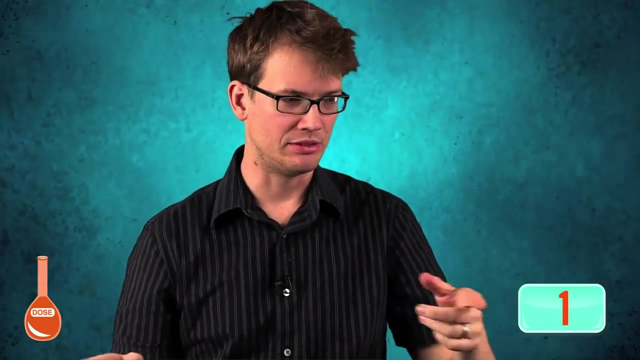 Who's hitting me in the face every single time. Okay, instead of the balls, we're just going to do a clock, because I get nosebleeds pretty easily and I don't want you to have to see that. Seven billion people. it's hard to actually get your mind around how many people that is. 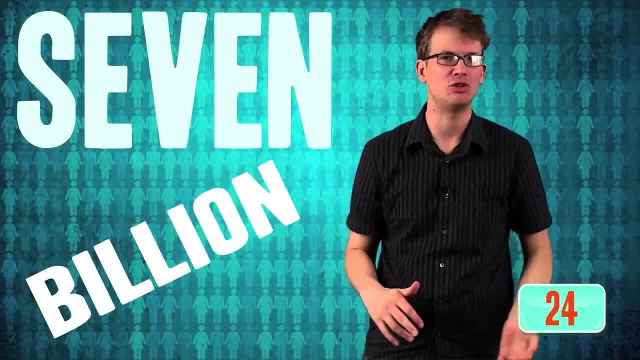 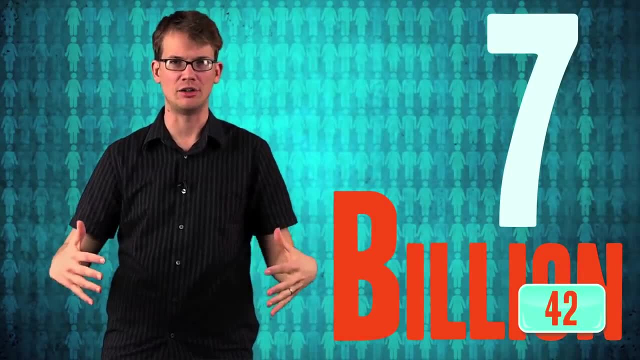 I mean, if we were going to just like sit down and count to seven billion, it would take you like 200 years or something. On the other hand, there is plenty of space for them If you took seven billion people and stood us shoulder to shoulder like we were at a Sting concert. 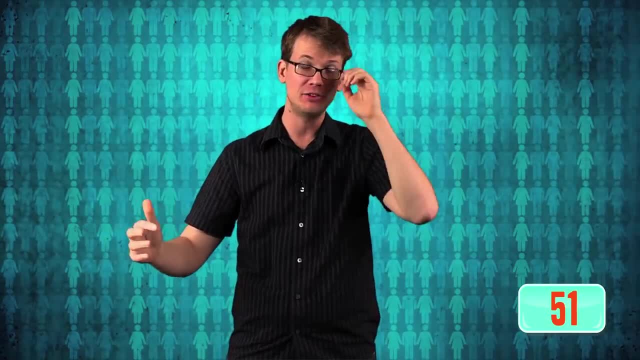 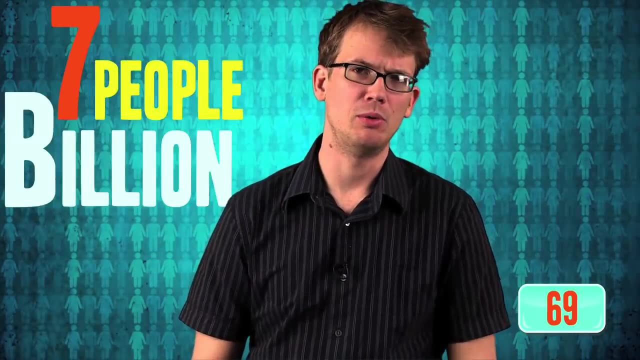 those seven billion people could fit in an area the size of Los Angeles. We can fit on the Earth. There's space for us all. So, as long as there's space for us all, what's the big deal about having seven billion people? 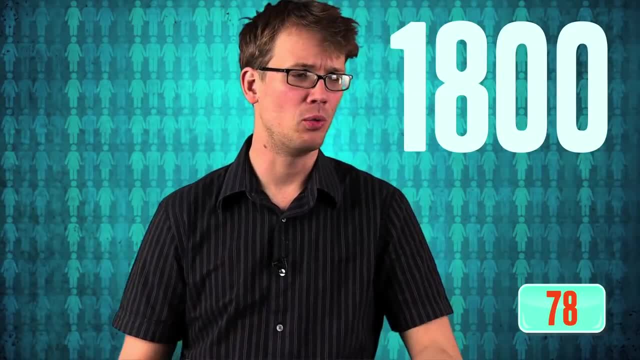 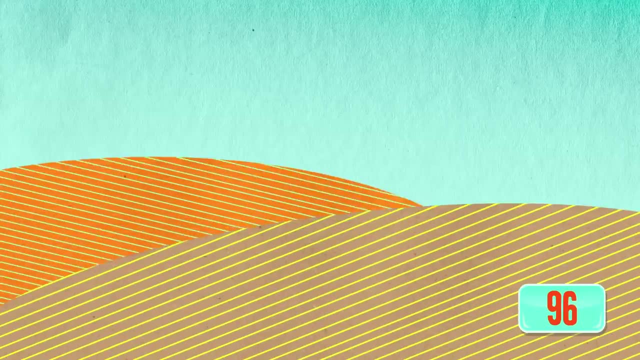 Well, it turns out, people have been thinking about this for a long time, since around 1800, when the world first clocked one billion people. I know what you're thinking: you're like one billion, that's nothing. Well, at that time, all the economies in the world were based on agriculture. 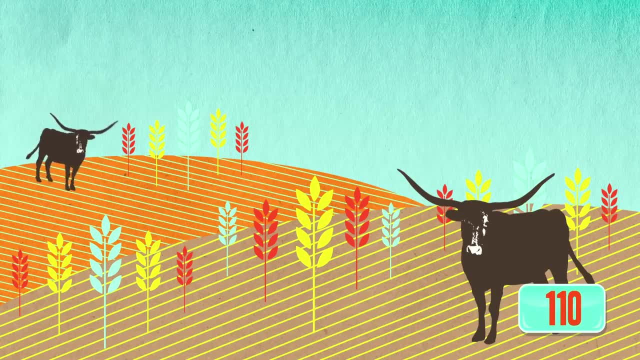 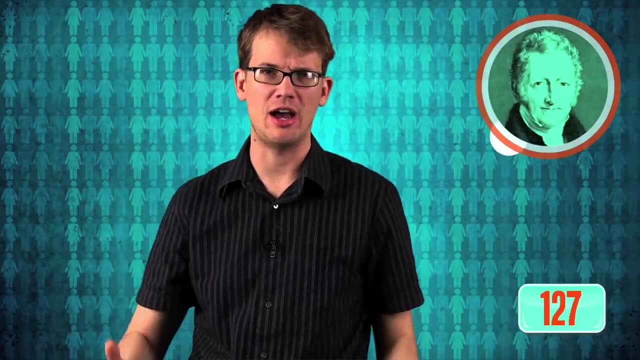 How much stuff we could grow with human hands: farm animals, maybe a scythe and a wooden plow or something, So that kind of technology. a billion people was really pushing it And the first like big-time thinker guy to. 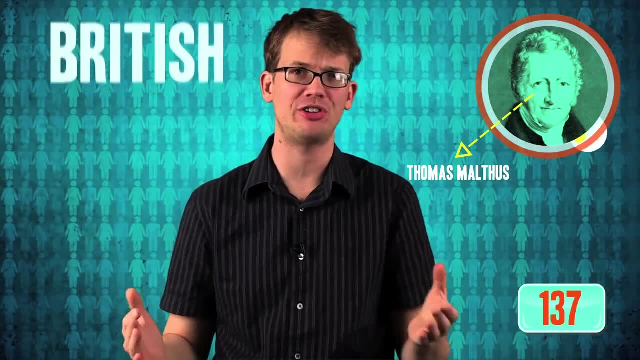 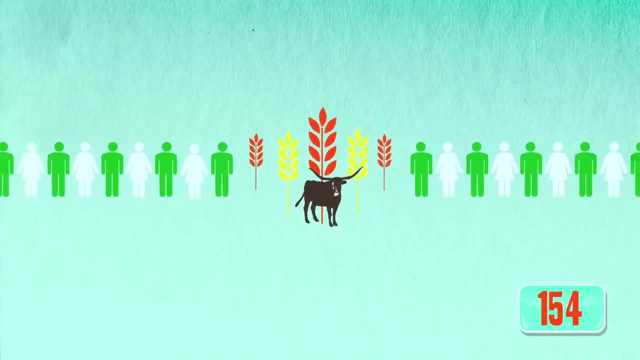 totally have a cow about there just being too many frickin' people- was a British economist named Thomas Malthus. Thomas Malthus calculated that human populations tend to grow exponentially, while the ability of humans to feed each other tends to grow more linearly. 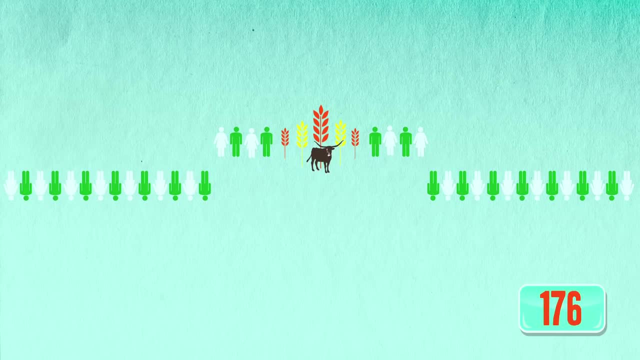 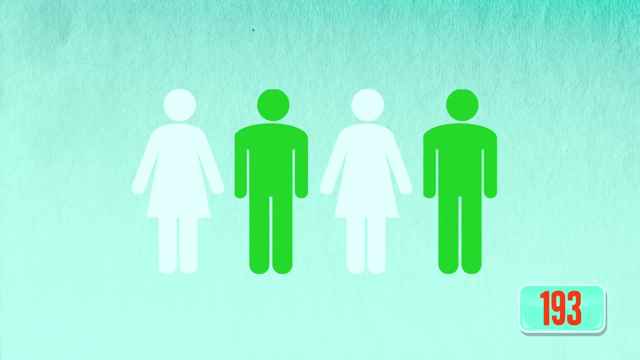 And so our growth as a species tends to outstrip our ability to feed everyone, And when that happens, it's pretty obvious what happens: You get the famine and the starvation, And for the people who are left over, who don't die of those things, they can get taken care of by disease and war. 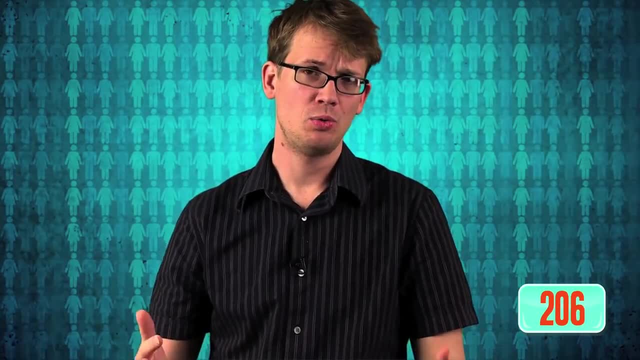 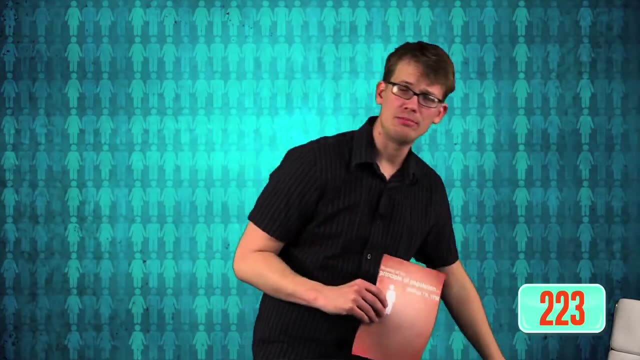 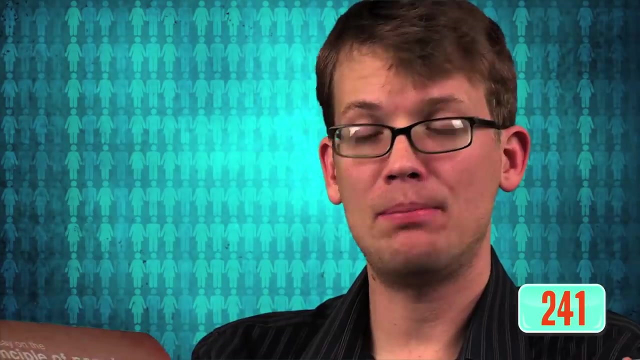 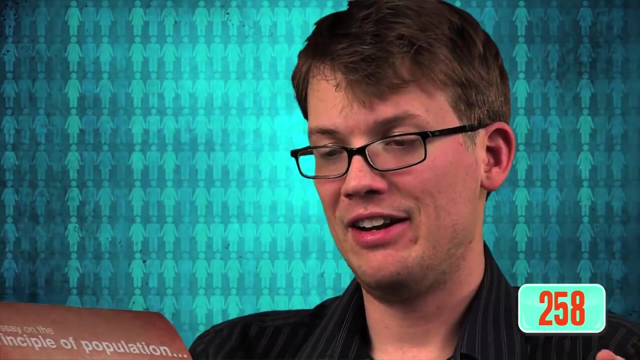 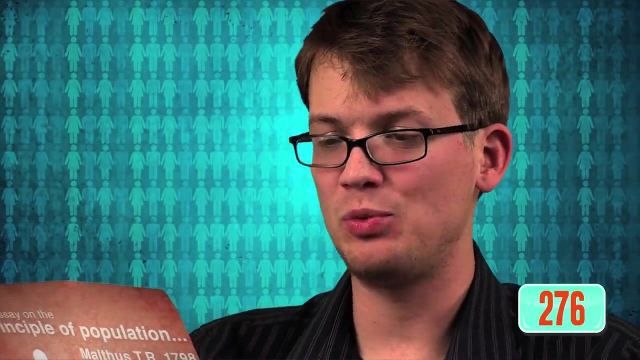 Basically, Malthus thought that humanity's natural date was to be cruel, miserable, pathetic and sniveling in a pile of dirty underpants. In his essay on the principle of population, Malthus observed their thousands and tens of thousands. Should their success be still incomplete. gigantic, inevitable famine stalks in the rear and with one mighty blow levels the population with the food of the world. Diseases also have an easier time taking hold and of course, starvation can kill an awful lot of people as well. 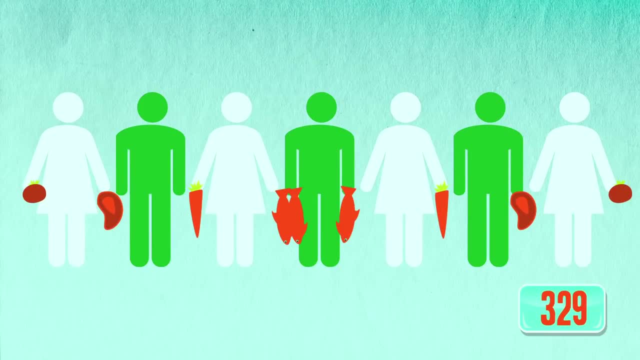 Though we did make some pretty good points. As long as humanity is well-fed, we're a pretty nice lot of people. But I have this problem too. When my blood sugar just gets a little bit low, I start killing all of my neighbor. That's not actually true. When you and your family's lives are threatened by starvation, there's a lot of things that you will do for food, including go to war. However, what Mr Doom and Gloom didn't predict was the frickin' Industrial Revolution. 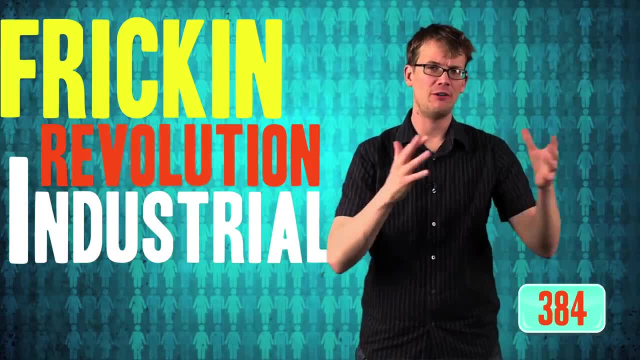 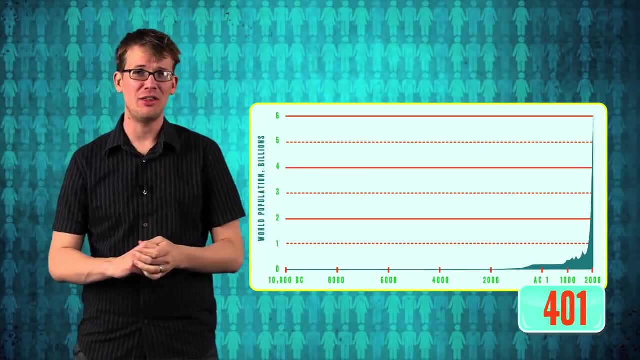 which not only allowed the production of much more food with far fewer laborers, it was also the impetus for this. Uh yeah, What that there is is, uh, the population of the Earth busting through Malthus's ceiling. 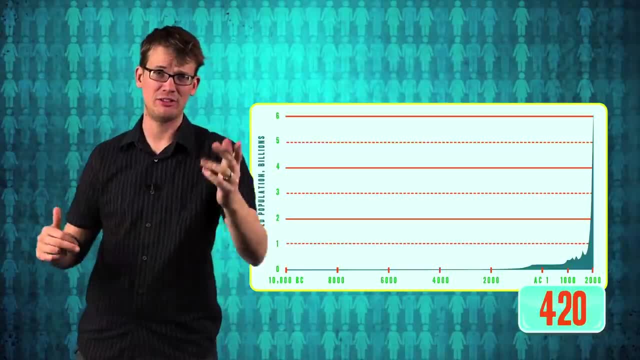 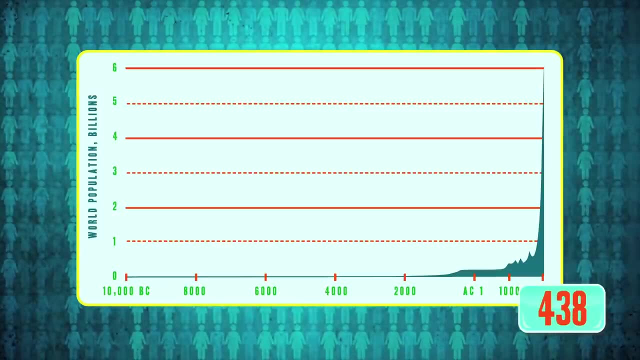 and then his atmosphere, and then his ozone layer, and then his mesosphere, and then his Probably be pretty impressed by this. If you're not impressed yet, uh, just keep staring at it. I can wait. I got all day. 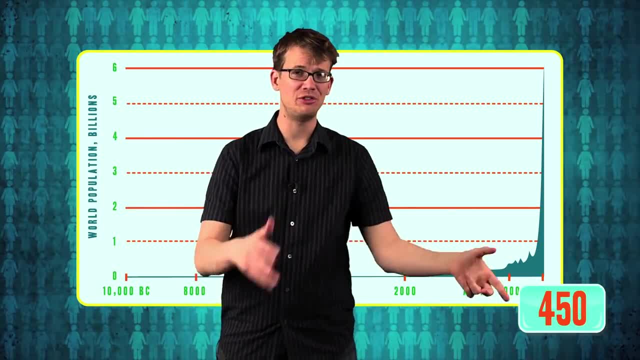 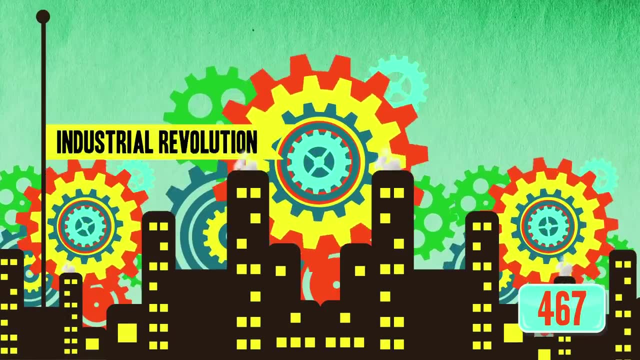 It took humanity 50,000 years to go from zero to one billion people and then to get from one billion to seven billion- about 200.. So wow, Industrial Revolution. thank you For allowing us to grow more food using machines. 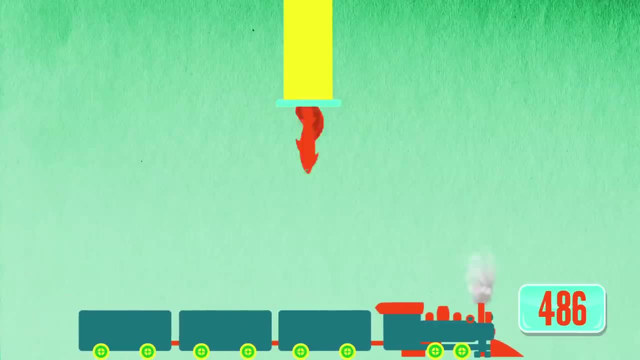 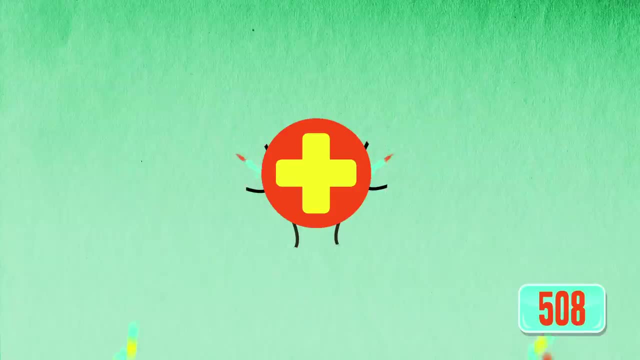 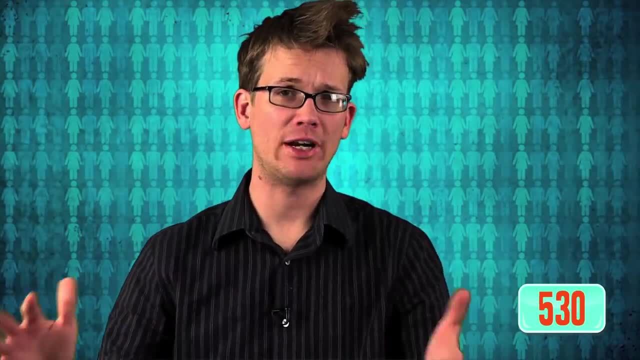 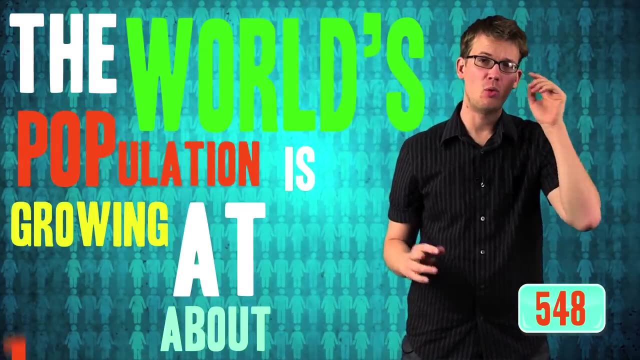 Yeah, industrial revolution. So Malthus might have been right about how frickin' stupid it was to be a human IF the industry Revolution had not happened. So now the world's population is growing about one-point-one percent per year. 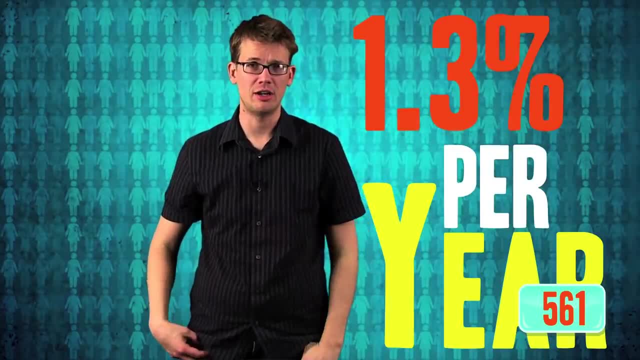 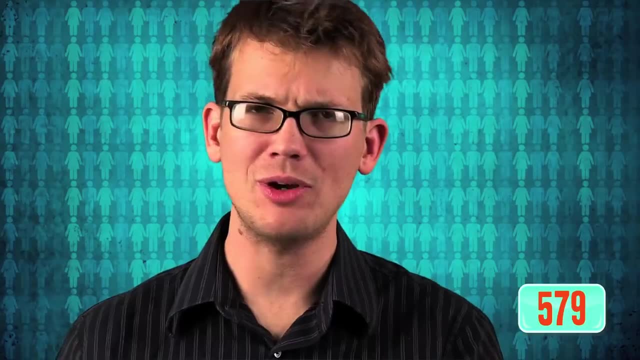 which is a tiny bit better than the one-point-three percent per year that got us here. If this current rate continues, by 2050, we should have about nine-point-three billion people- people on the planet. So the question is, at what point are these numbers going to outstrip? 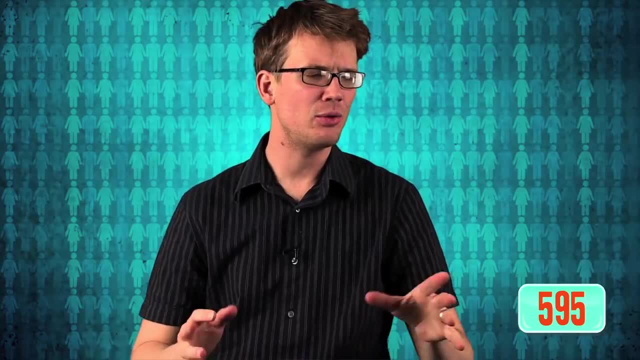 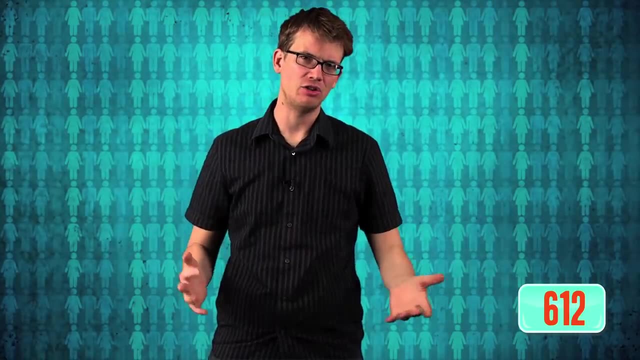 our ability to feed all of the people on the planet. It turns out, actually, that the question isn't how many people can the Earth accommodate. it's more like how many rich people can the Earth accommodate, Because people in general, they tend to demand stuff for their survival. 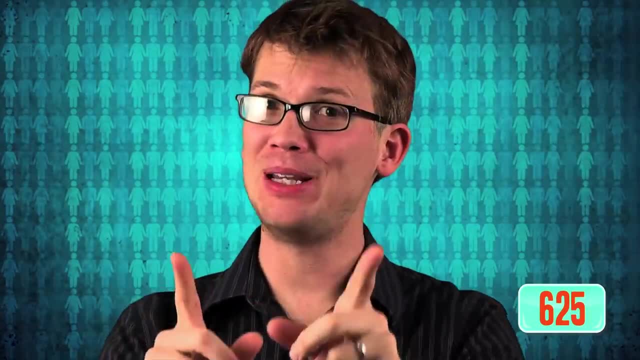 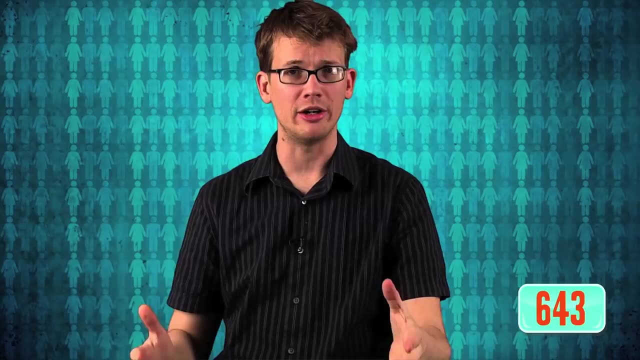 like oxygen, water and food, But rich people. we have different expectations. We, for example, in America, have a lot of agricultural crops and we have to use a lot of fresh water to water those agricultural crops. Do you wanna take a guess at the number one irrigated crop? 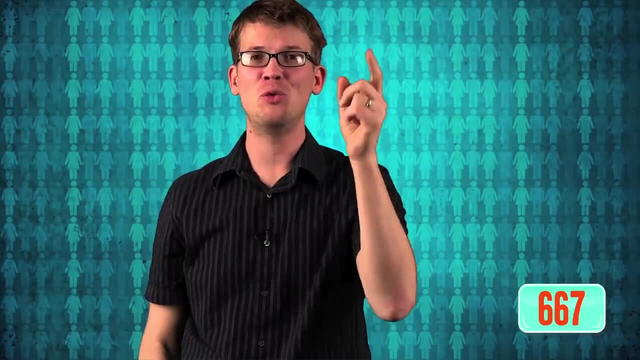 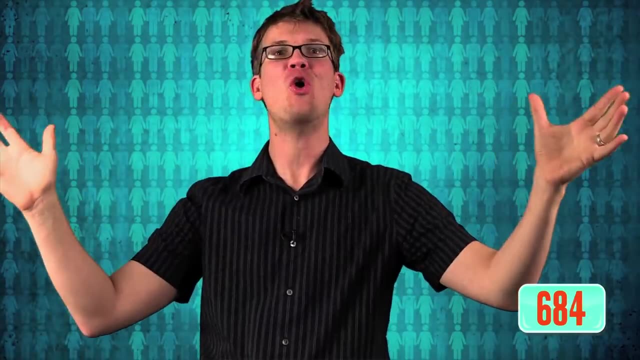 in the United States of America. Unless you've heard this statistic before, you were wrong. It's grass. It takes more water to create lawns than it does to create all of the corn in America. We're using it like crazy, though it is a pretty scarce resource We can use. 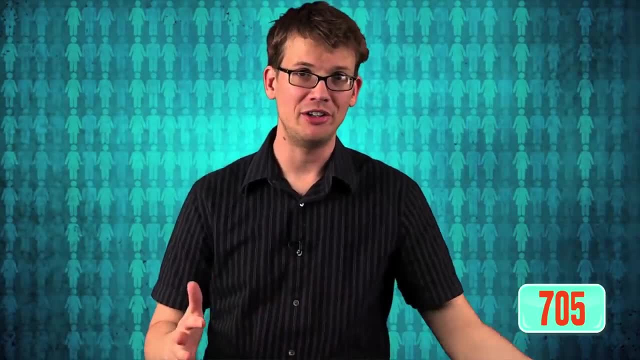 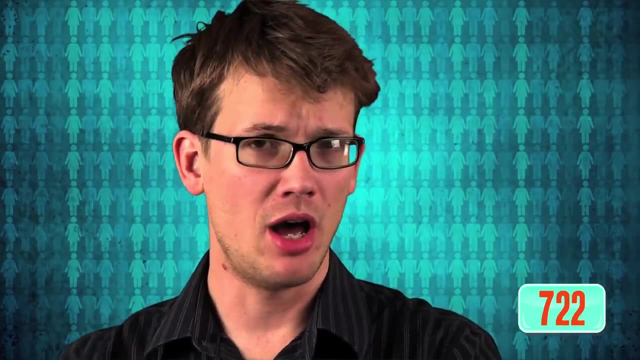 less than one percent of the water on our planet. Most of it is salt water that we cannot use to drink or irrigate crops, and seventy percent of our fresh water is frozen in glaciers. So clean fresh water, non-negotiable and scarce. So what's next? Uh, food, The world's. 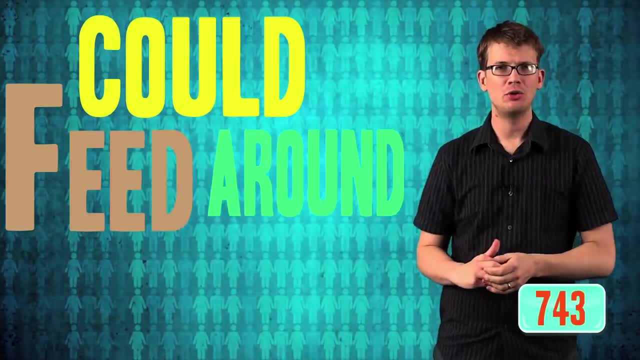 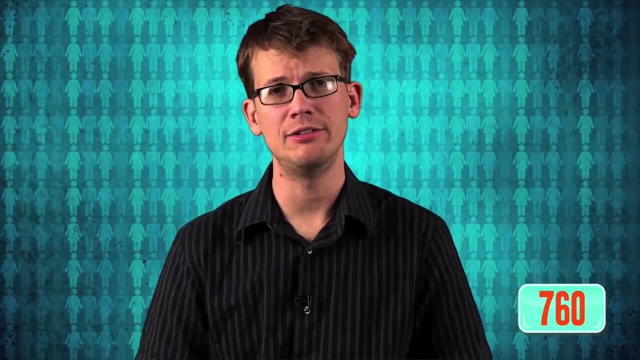 combined food output could feed around eleven billion people, and yet there are one billion people who need food. So yeah, that's one of the most pathetic and infuriating things about our planet. So if there's enough food for eleven billion people- and there's seven, 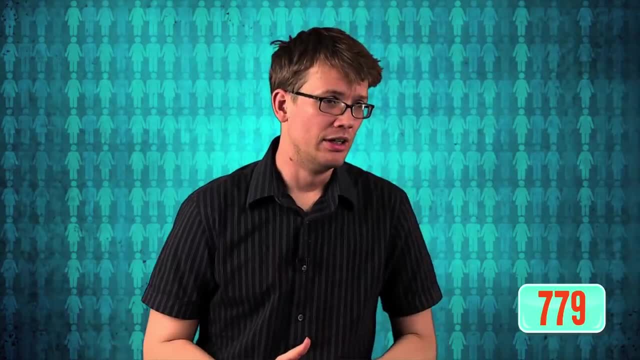 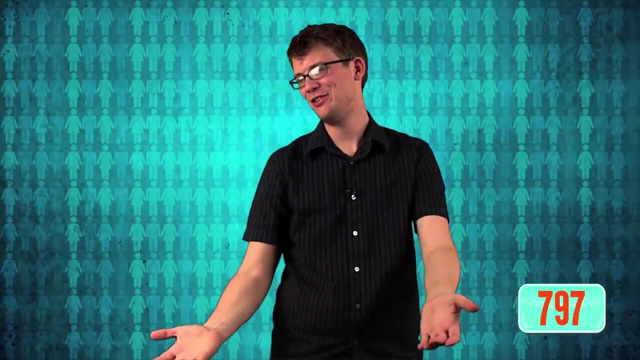 billion people, and a billion of them are hungry. who is eating all of our food? Food is eating all that food. A huge amount of the food that we grow in America gets, uh, in turn, eaten by livestock. It's so hard to say the truth, which is that, but rich people can do what they want. 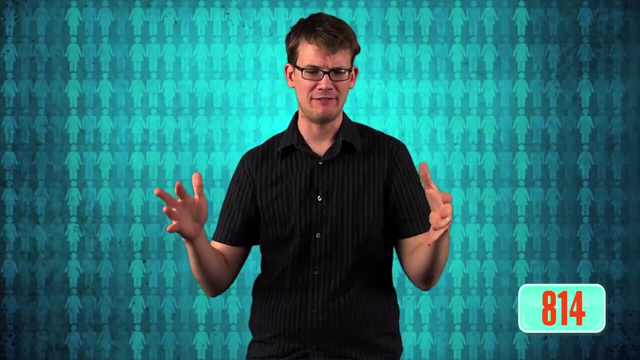 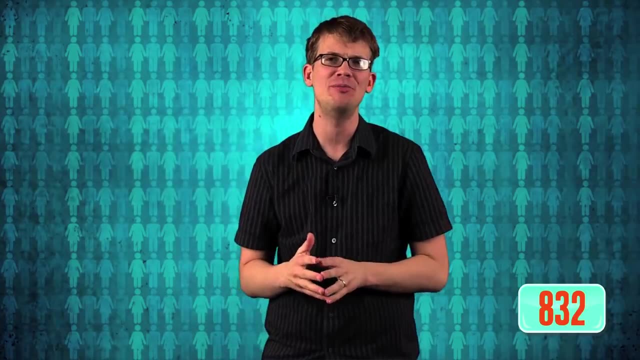 Now, when I say rich, it's important to note that I'm not talking about, like, uh, the ninety-nine percent versus the one percent rich. I'm talking about if you have running water, electricity that comes into your home, a computer that you can watch YouTube videos. 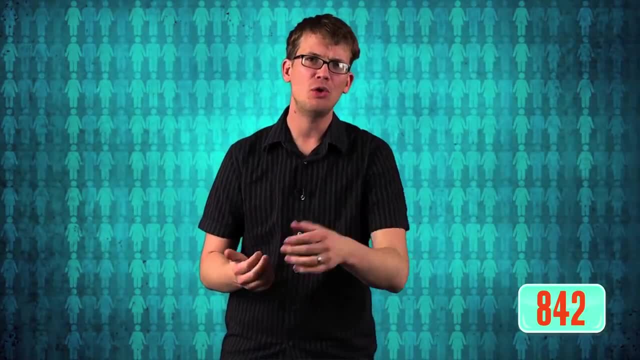 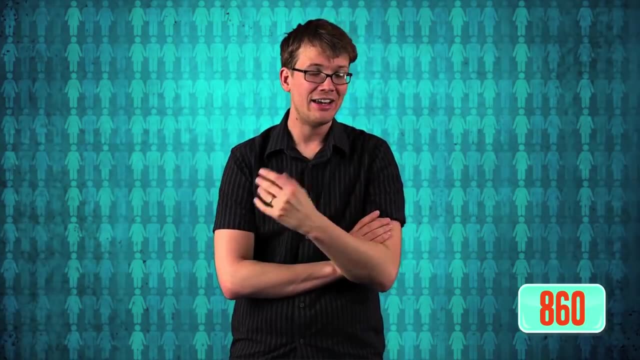 on and regularly, uh, can afford to eat meat. you are a rich person On the earth And, and you know, sometimes we just have to come to terms with the fact that we, even those of us who don't have it great in America, have it better. 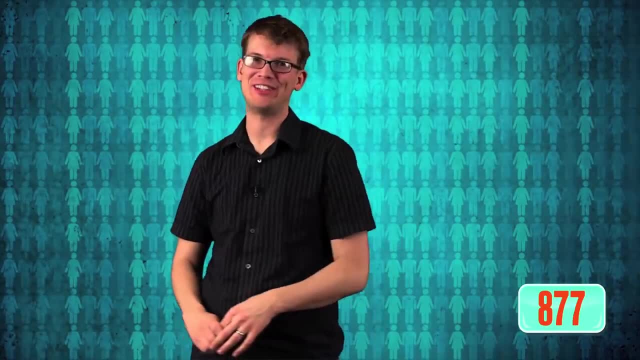 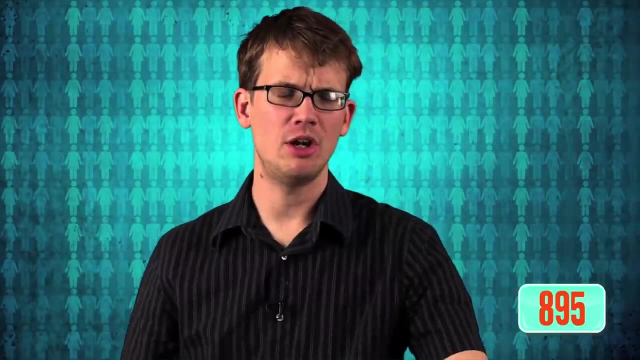 Better off than a whole lot of other people. There's a lot of people in the world who don't get that. If you can have a hot shower, that's like the peak of luxury to me. So, assuming that you are a first-worlder, that you live in a developed country in Europe or you live, 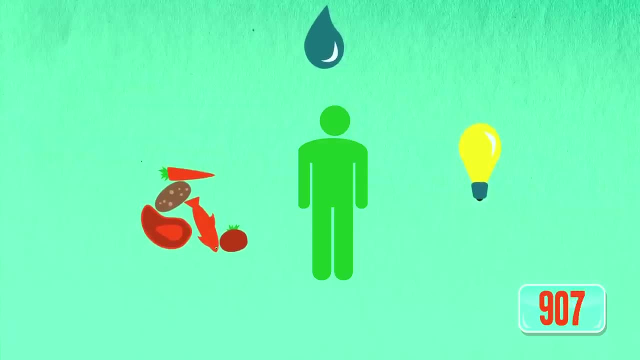 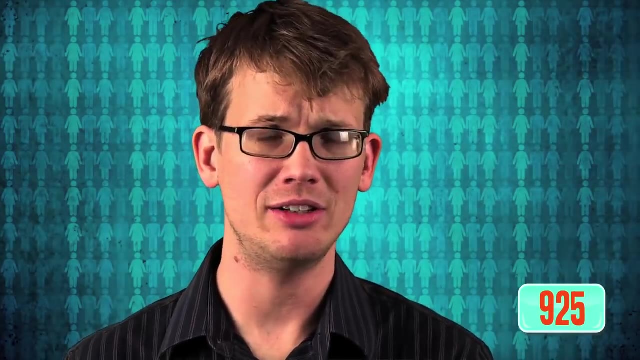 in America or Japan, you consume, on average, as much stuff as thirty-two Kenyans. And now the number of well-off people in the world is starting to increase dramatically and quickly, and this is what we've always wanted for the world. 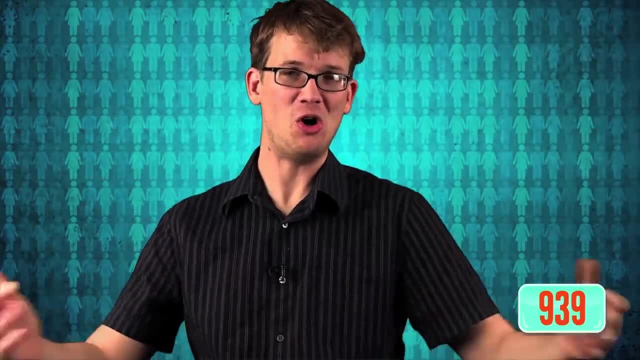 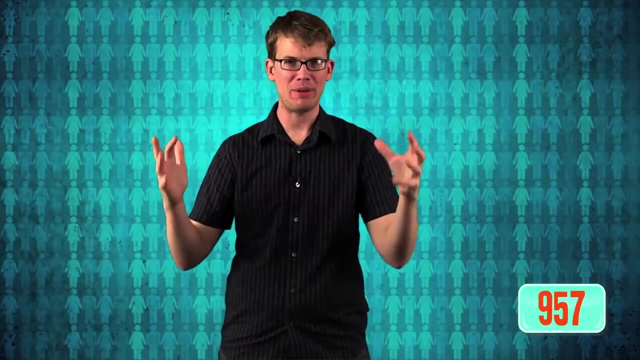 So now we have all these moderately well-off people walking around all over the planet, which is great, except that they require more. In the meantime, though, a huge percentage of all of the babies that we're talking about being born right now aren't being born to these rich people in the developed world. They're being born in developing nations, and so the population isn't just growing. It's growing in this weird sort of scary lopsided way. In fact, just people in a lot of developed countries have kind of stopped having babies, Like Japan, for example. Everybody's. like Japan. what are you doing? Why aren't you having any babies? And Japan's like? I don't know, I don't feel like it. They're having about one baby per household. They're not even replacing themselves compared. to two or three babies in America, or like five or six in most of sub-Saharan Africa. So developing nations are having a baby boom and that's what happens. when you get, you know, vaccines and antibiotics and safe water and better sanitation, You get fewer babies. 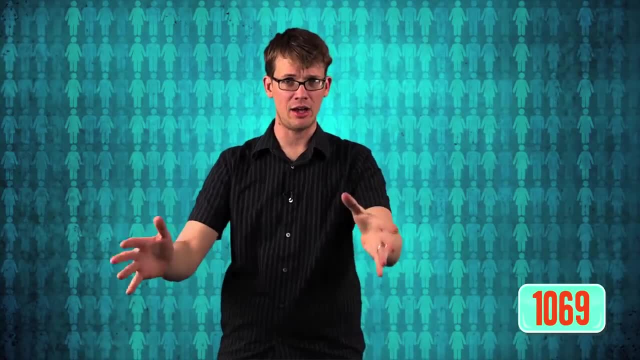 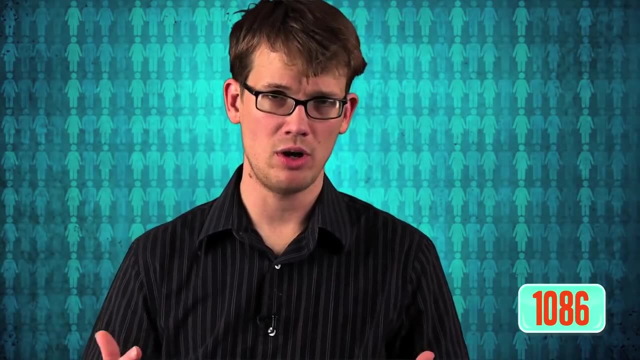 dying, and we are all completely and totally in favor of fewer babies dying, I hope. But it also means that there are going to be a lot of new sub-Saharan Africans in the next fifty years or so, and that is where a lot of the one billion currently hungry. 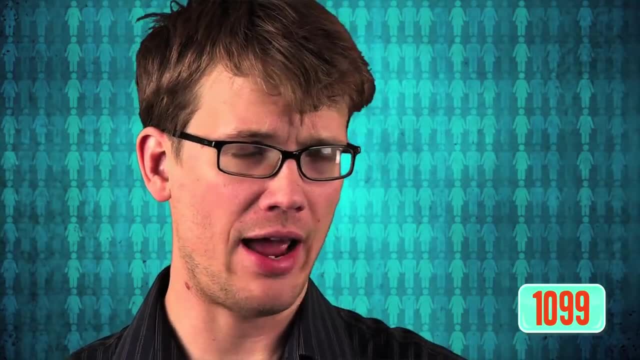 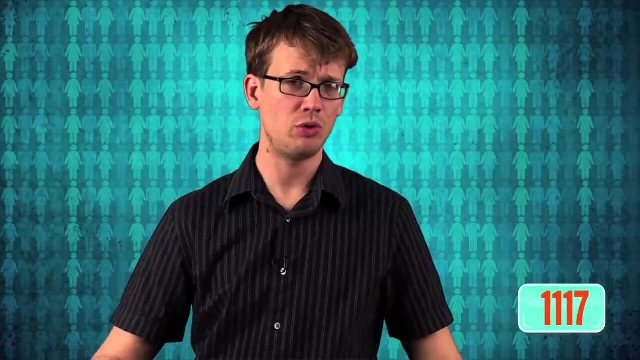 people are already living, And while those of us in the developed world are not having any babies at all and yet consuming enough food for like four truckloads of babies, the governments of developing countries are struggling with where to put all of these new people and how to feed them all. 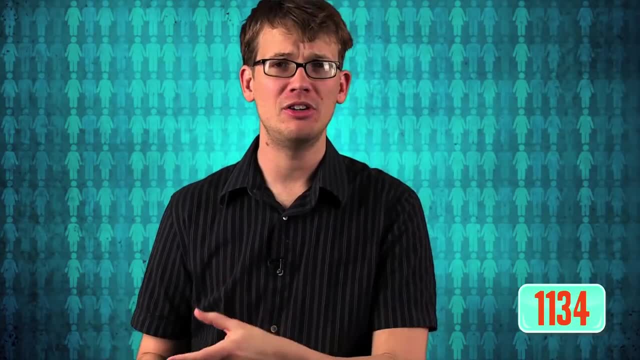 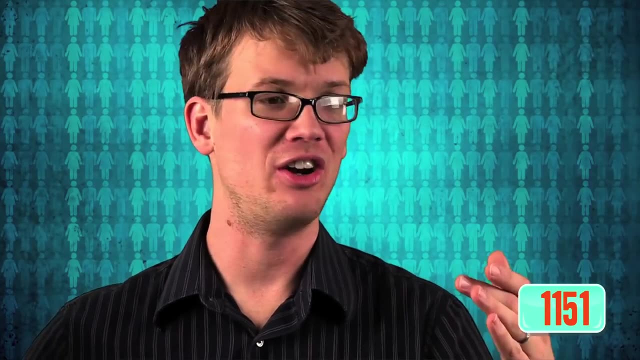 And you also get what is known as a youth bulge. A lot of developing nations are currently seeing a huge explosion in people between the ages of 15 and like 29. And all those youth are out there looking for the same jobs, all at the same time feeling generally hormonal. 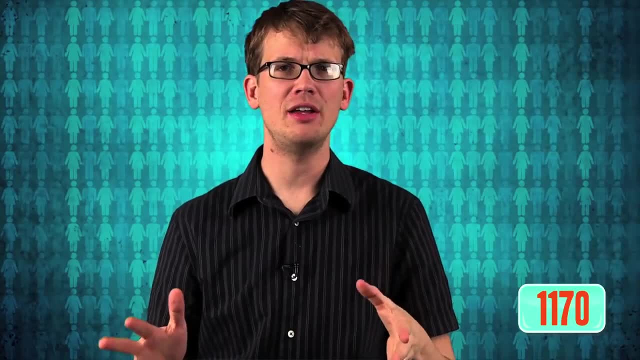 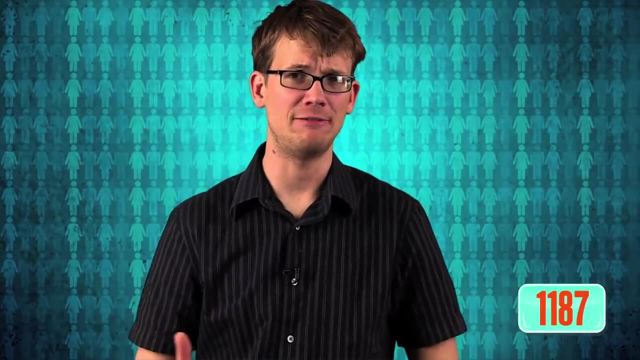 as youth do, and being pretty unhappy with their lot in life. Some social scientists conjecture that youth bulges like this have been responsible for nearly every insurrection in history, from the English Revolution in 1640 to the more recent Arab Spring, And neither of those things were bad things. but we should be aware that.